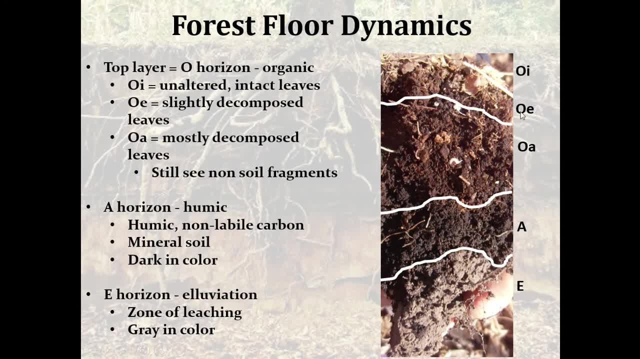 you're interested. it's categorized by the OI, OE, OA, and then we move into the A horizon and then we have an E horizon in this picture as well. So the different subhorizons are just how decomposed the organic matter is, And it moves from unaltered, readily distinguished material. 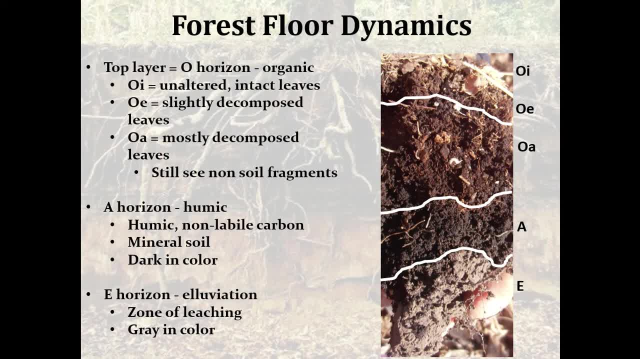 all the way down to mostly decomposed leaves. but we're not seeing any mineral content until we get to the A horizon. That's where we have our humic, non-layable carbon. we'll get into what that means more later, but it's a mineral soil, dark in color. Our E horizon is where 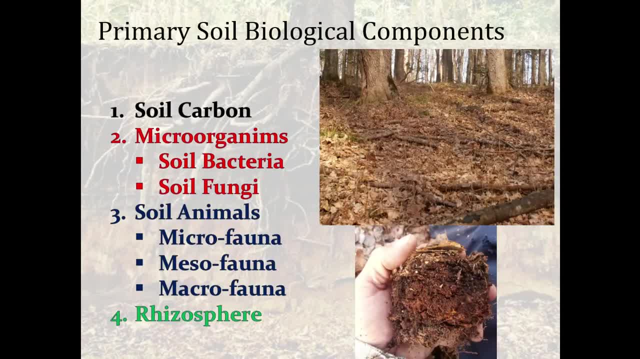 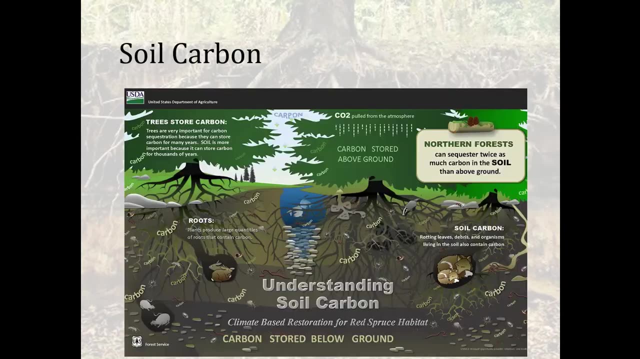 a zone of bleaching, usually lighter in color, often gray. So primary soil biological components is the soil carbon, then our microorganisms, our macro organisms, our soil animals, and then we'll talk about the rhizosphere. So soil carbon. soil carbon drives a lot of our 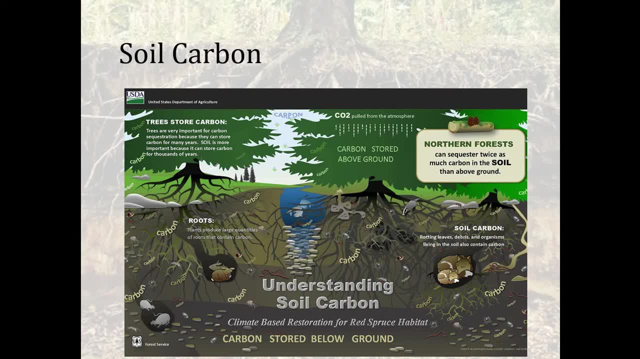 nutrient availability for plants and animals. the importance of forests in the role of soil carbon. A little note here that forests are able to sequester twice as much carbon below the soil than they are above it. So a lot of times we think, oh, we need to grow. 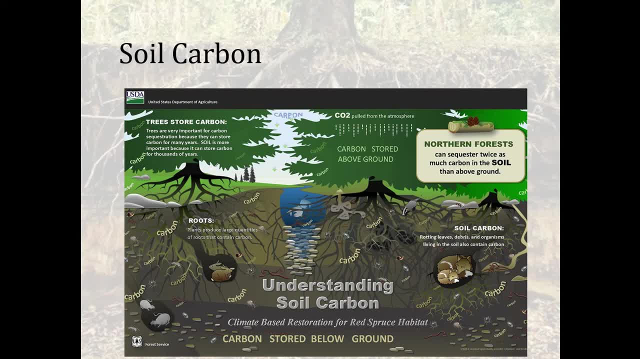 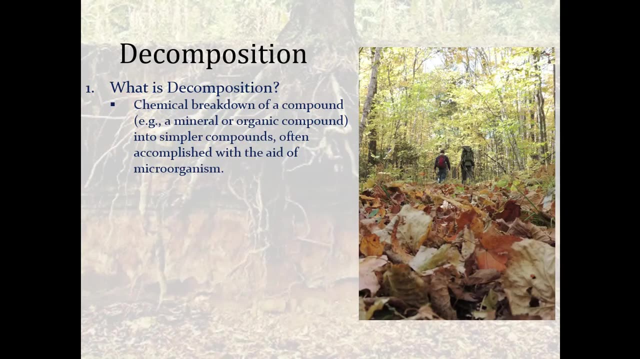 more trees, grow forests. stop cutting down our forests. but it's really their ability to store that carbon in the soil for long-term cycling down there that is also really important when it comes to carbon sequestration. So, decomposition of organic matter First, we 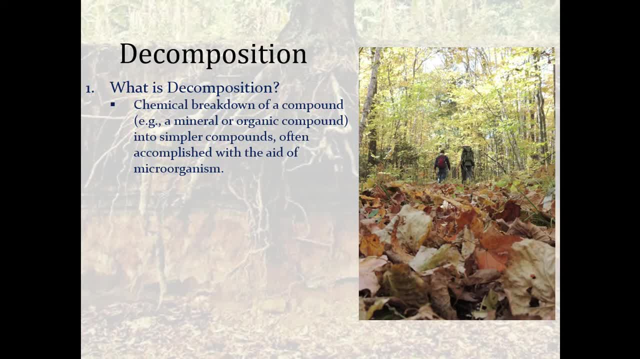 start with, what is decomposition? So it's the breakdown of a compound into simpler compounds. So I think of like a really long carbon chain. When it gets decomposed it forms like two shorter chains and so on and so forth. It's a simplification of structures, often for the gain of microorganisms Eventually. 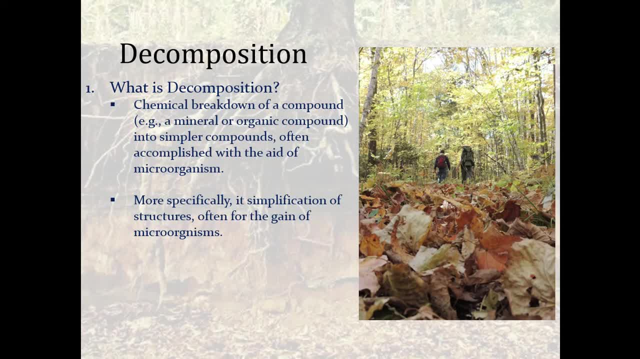 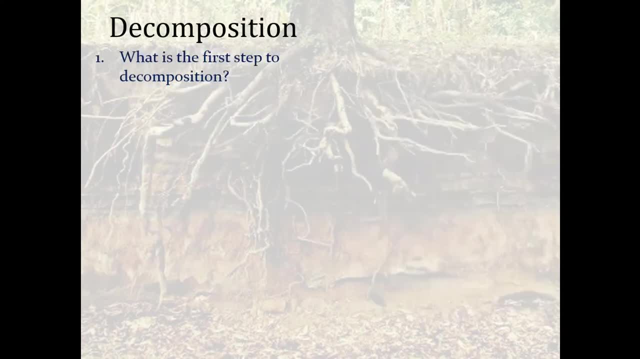 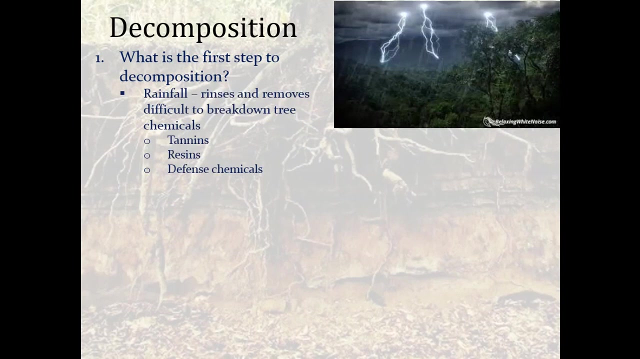 these microorganisms decompose to the point that the plants can then use those nutrients again as well. Okay, So does decomposition only occur from living organisms? We will find out: The first step of decomposition: rainfall. So there's our answer: Rainfall, not a living organism, but 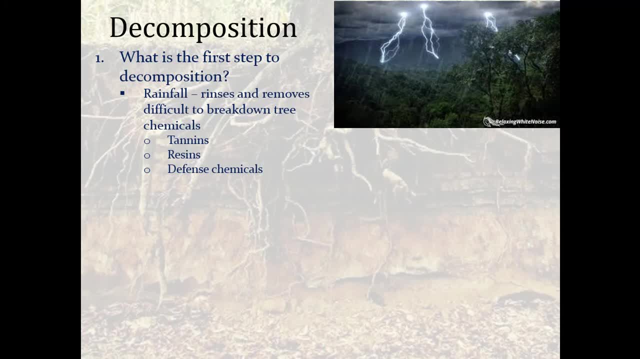 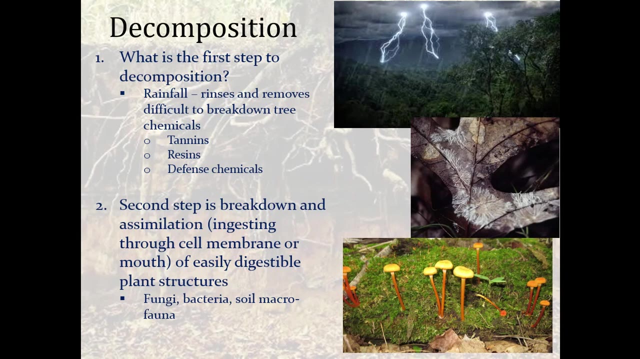 really important for decomposition, for the material to get wet as well as rinse away some of those tannins and other defense chemicals from the soil, The tree components, especially the leaves. Then the second step is assimilation, or the ingesting of a cell membrane through a mouth or easily digestible plant structures. So 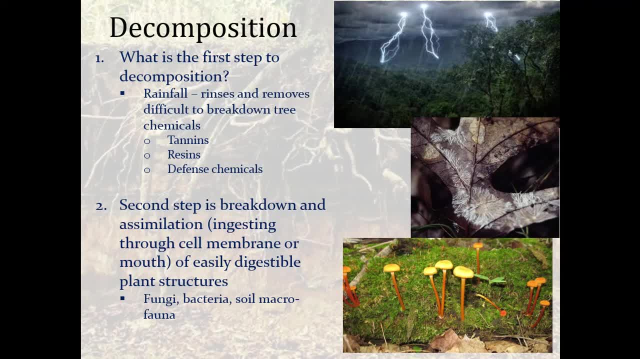 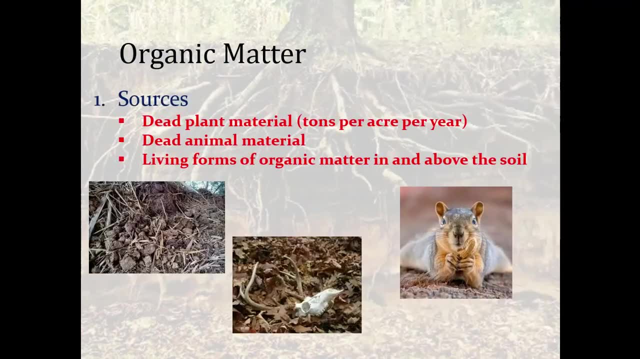 fungi, bacteria, soil, macrofauna are beginning to break down the cell membrane and break those long carbon chains into shorter components. Okay, So we're going to look at sources of organic matter. Probably most often think of dead plant material, So this is just naturally cycling material. We also have dead animals. 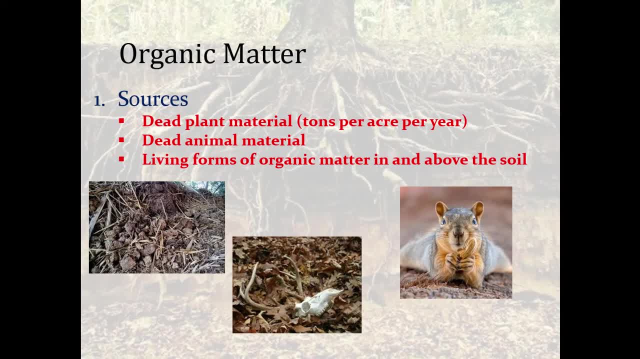 in there In a more natural setting. think of those carcasses and things come to feed on them. but there's always some part of it left in the soil or from animal waste that is being broken down, And then there's living forms of organic matter in above the soil. 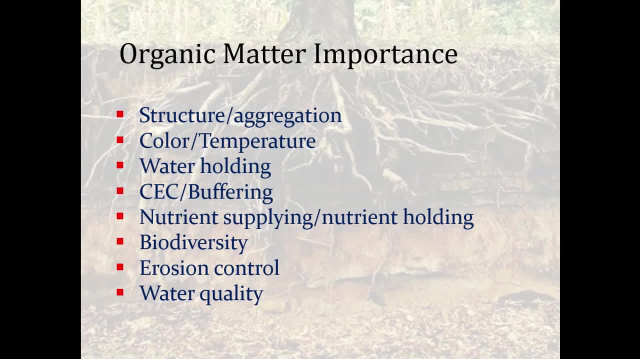 This would be our plants: The importance of organic matter- we mentioned it in some previous videos- for soil structure and aggregation, color, water holding capacity, cation exchange capacity or nutrient supply and holding biodiversity in our micro and macro organisms and plant communities. And 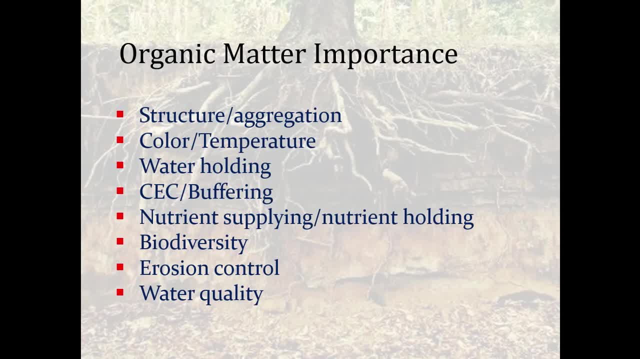 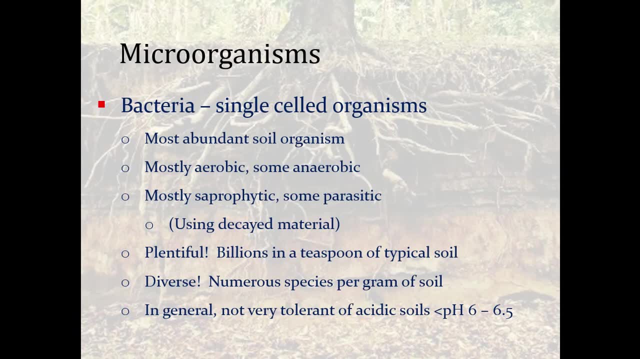 then both of those drive erosion control and water quality, so water filtering as well. Microorganisms, Microorganisms, Microorganisms are. we have our bacteria, which are single-celled organisms. These are the most abundant soil organism, mostly in aerobic conditions. Some do operate better. 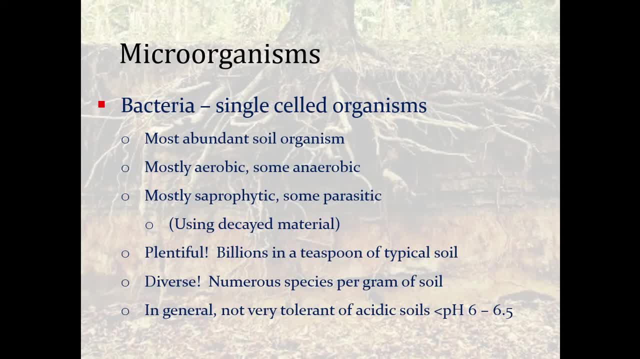 in anaerobic. Remember aerobic means in the presence of oxygen. Anaerobic is when there's a lack of oxygen available, Mostly saprophytic, but some are parasitic. And here a reminder that saprophytic means that they use decaying material. 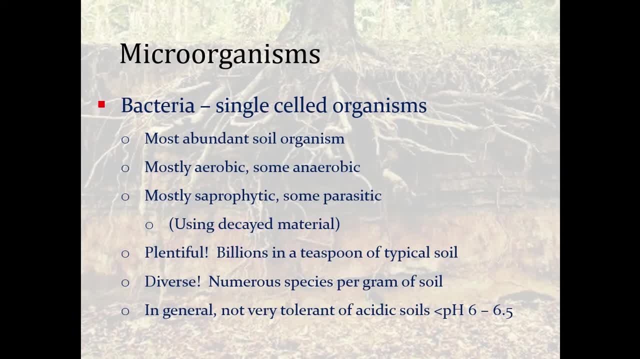 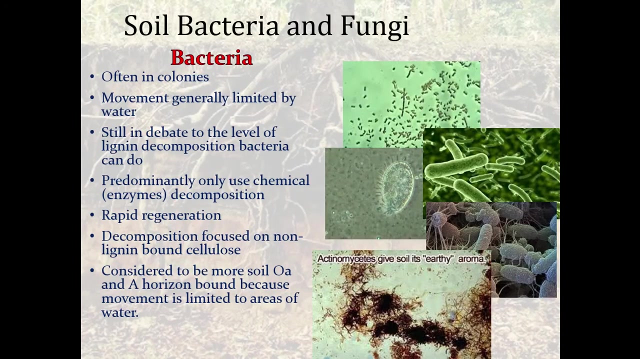 Parasitic would mean that they feed on living material. Bacteria are incredibly plentiful and diverse in the soil, but in general not very tolerant of acidic soils. So as we get below pH of 6.5 to 6, we lose a lot of our bacterial communities. 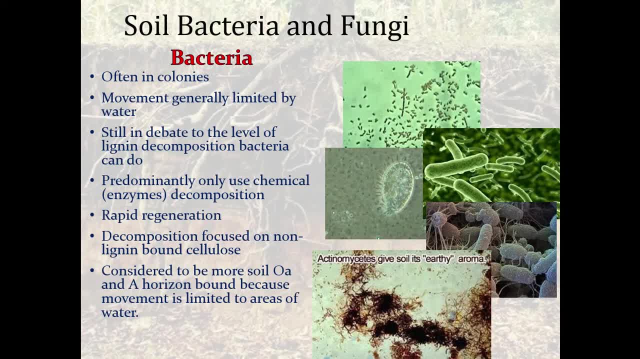 While they are single-celled organisms, they often form colonies and move through the use of water. They predominantly use chemical decomposition and feature rapid regeneration. So when conditions are right, your bacterial population can quickly grow and sort of use all of those conditions that favor them, Mostly found in like the OA A-horizon, because their 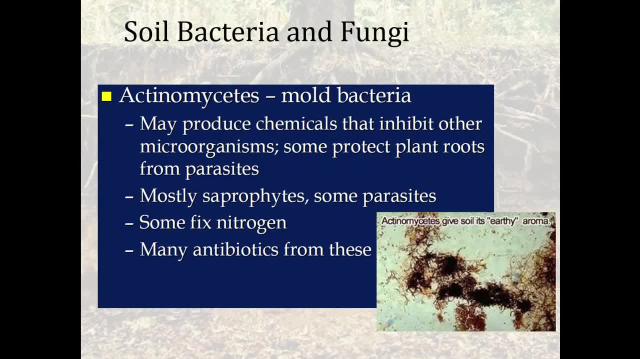 movement is limited by water. Actinomycetes or mold bacteria is just one subcategory of bacteria, But we highlight it because it produces chemicals that inhibit other microorganisms. Some of those chemicals then protect plant roots from parasites, So sort of a symbiotic relationship going on. 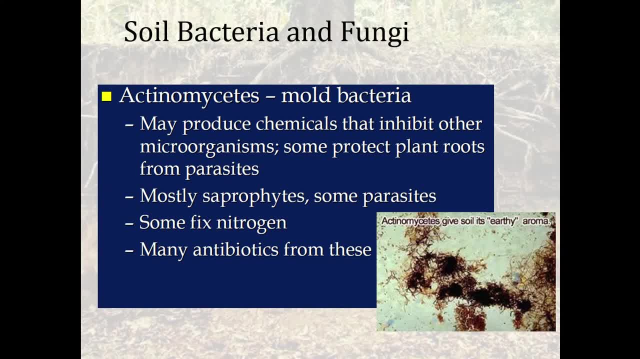 here. These are also some of them that fix nitrogen in the soil. And then many antibiotics come from mold bacteria And we talked about In the intro video the importance of soil bacteria for development of pharmaceuticals. So this is a family that they research and look for and test for future drug development. 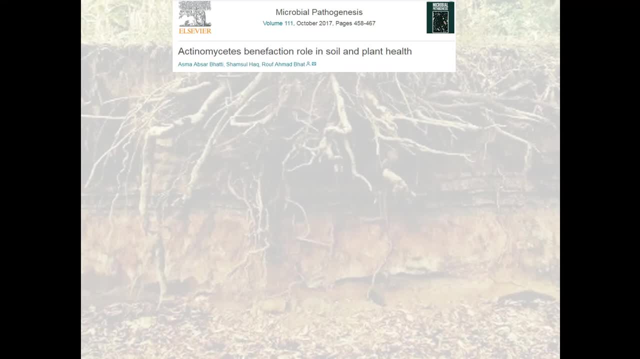 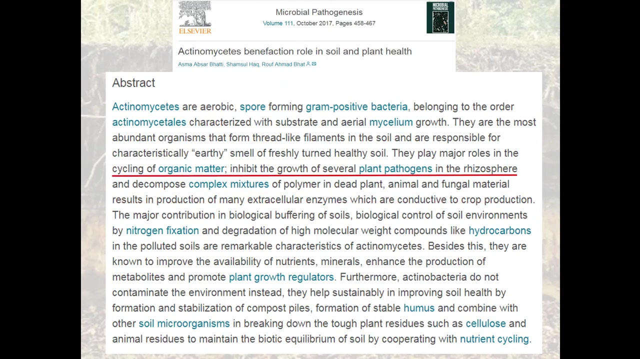 If you want more reading, here's a really good paper on Actinomycetes. Benefit in Soil and Plant Health And just highlight: cycling of organic matter, inhibit several plant pathogens, improve crop production and then improve availability of minerals, nutrients and metabolites for 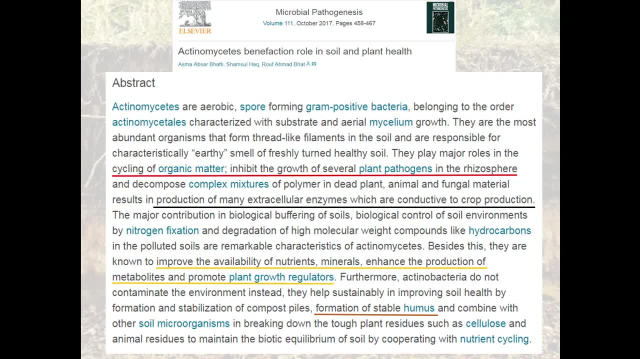 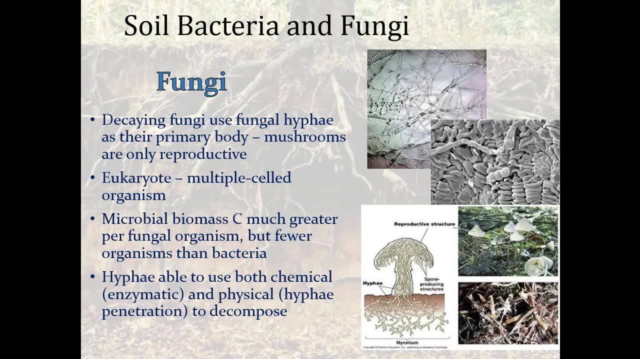 plant growth regulators, as well as form stable humus, And we'll talk more about humus in a later video. We also have fungi in the soil, So decaying fungi use hyphae as their primary body. These are sort of like roots. it's an. 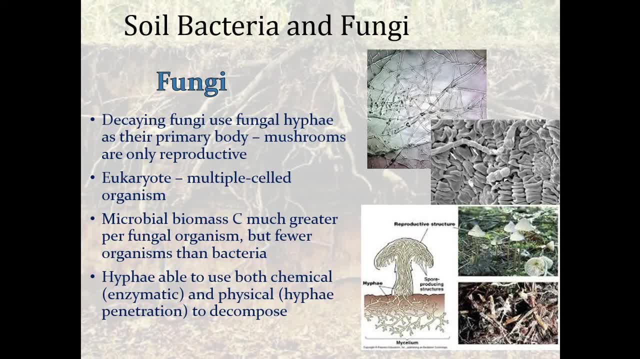 easier way to think of them, although they function differently, But these root structures in the soil, And then when we think of fungi, we always think of the mushrooms or shell fungus, things like that, But these are really just the reproductive body parts of them, And so a lot of times 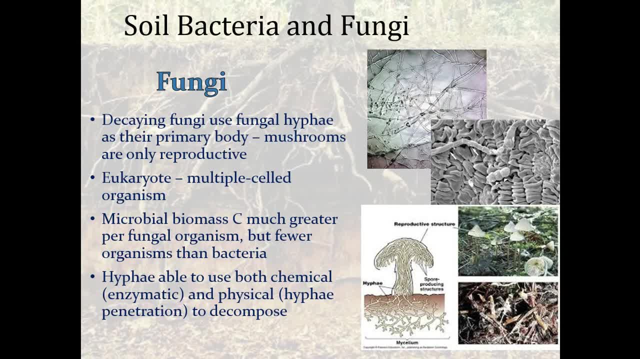 more mass below the soil that we're not seeing. so there's something to keep in mind. They are a eukaryote, or multiple-celled organisms. The carbon is much greater per fungal organism, so an individual organism is much larger. 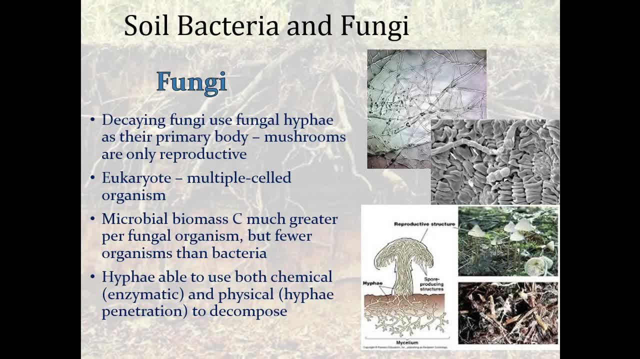 but the flip side of that is that there are fewer organisms than bacteria. If you think of bacteria, a single-celled organism forming a colony, that colony can be large, but that organism itself is sort of limited to that. single cell. Fungi are also capable of both chemical and physical decomposition, so they can penetrate. 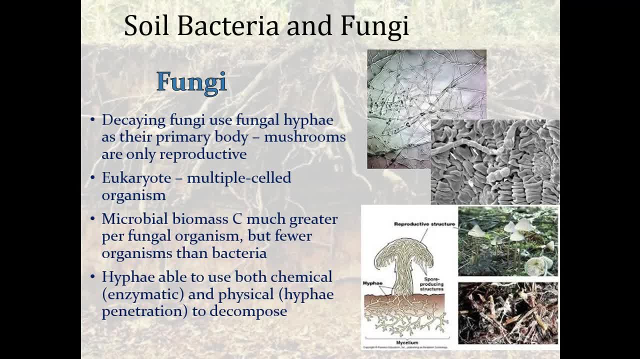 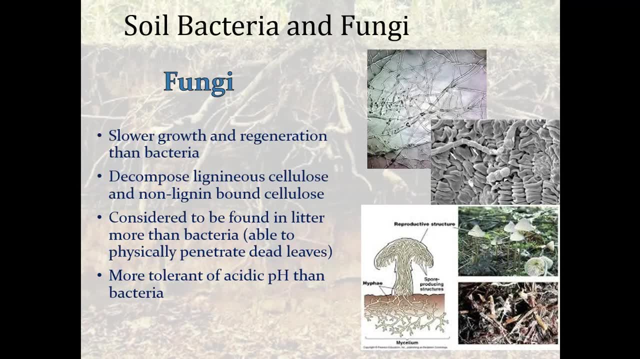 materials using their hyphae. Slower growth and regeneration than bacteria, but more longer-living, And they can decompose both lignin and non-lignin by found cellulose considered to be found in litter more than bacteria. So again they're able to penetrate dead leaves. they're able to spread broader and deeper. 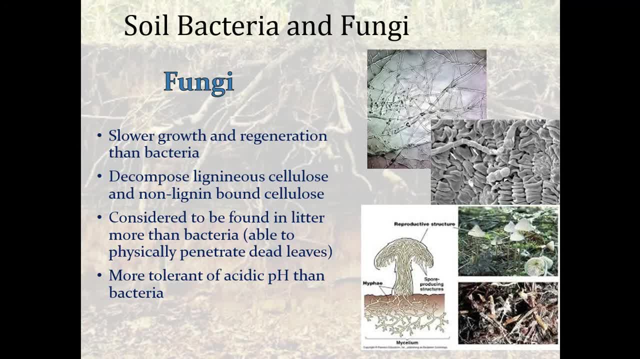 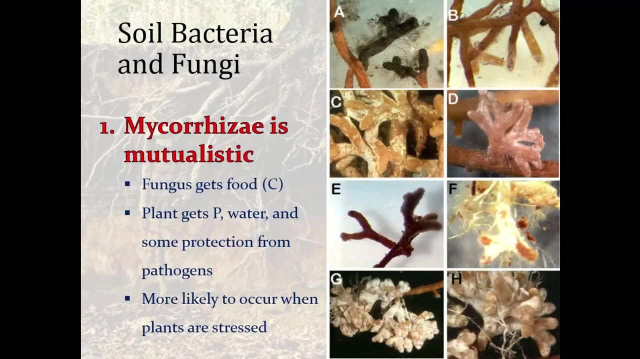 in the soil profile, as well as being more tolerant of acidic pH than bacteria. So a lot of times our forests are fungal-dominated due to that long, slow growth and being more tolerant of an acidic pH. Okay, Mycorrhizae fungi form a mutualistic relationship with plants. 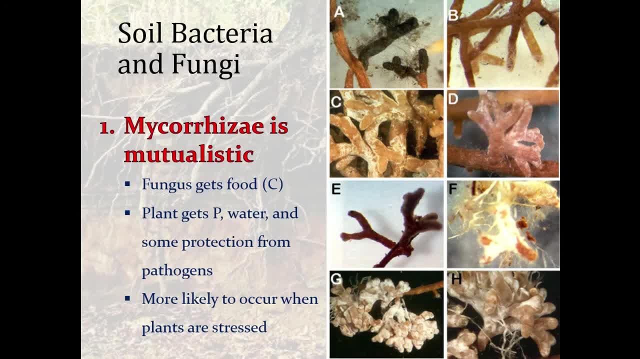 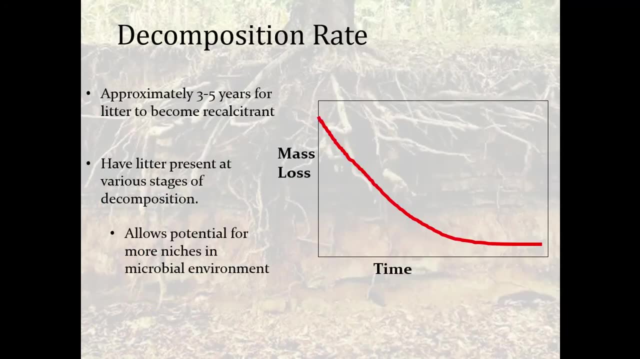 So the fungus gets carbon, the plant gets phosphorus water, maybe some protection from the pathogens. They also serve to exponentially increase the surface area of a plant's root system to acquire all those other resources. Decomposition rate: so approximately three to five years for litter to become recalcitrant.